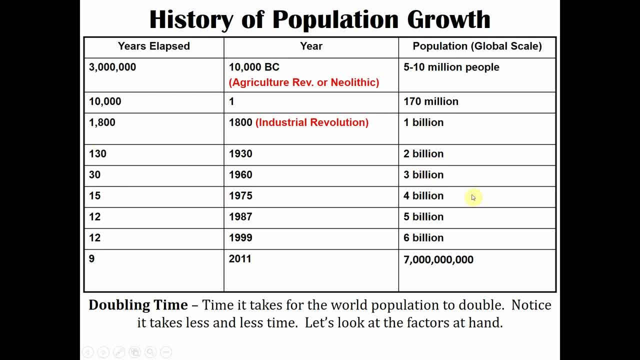 Three years, two to three, 30,. three to four. So you'll see it takes less and less time to get a billion people And that's indicative of better health care and better food. So let's look at those factors. The top left in the red you have the medical factors. 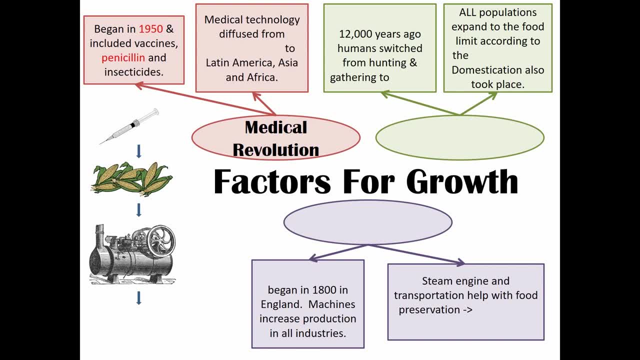 It begins in the 50s with vaccines and antibiotics and insecticides- Things that stop malaria, cholera and all of these diseases. It diffuses from the core to the semi-periphery and periphery And it's still spreading today. 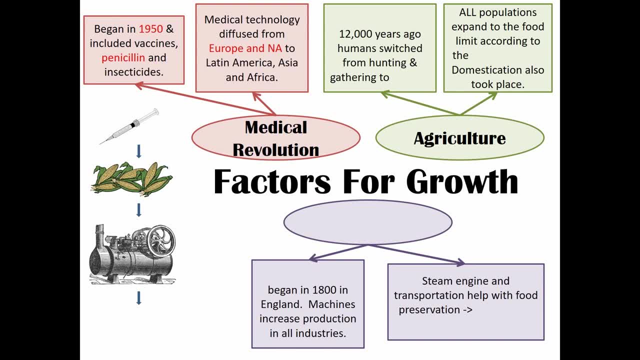 In the green, in the top right, you have agriculture. This is probably the biggest, because you can't grow if you don't eat. My son knows that right. So the Neolithic revolution was about 12,000 to 14,000 years ago. 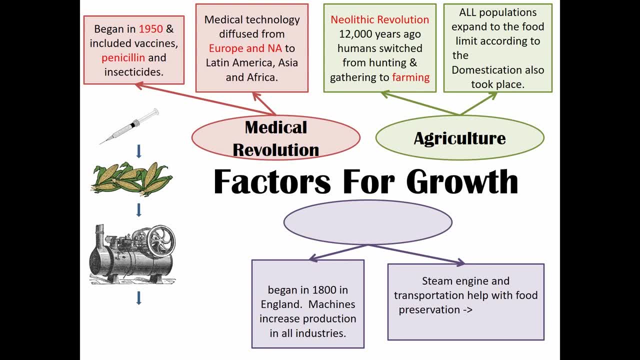 People switched from hunting and gathering and start farming- Not super efficient, but a massive upgrade. They also will start to domesticate animals. In the bottom we have the technology, And the industrial revolution is so key to that. We see that the steam engine produces. 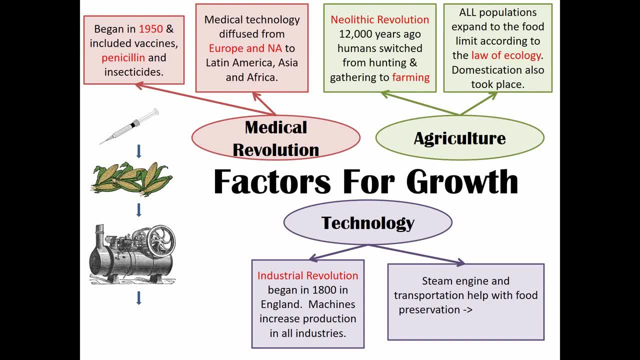 We have all these innovations, with factory mass production, Just tremendous amount of growth. And now we have more work being done by machines and less work being done by humans. So if you add all these together- right- medicine, food and machinery- you have ding ding. 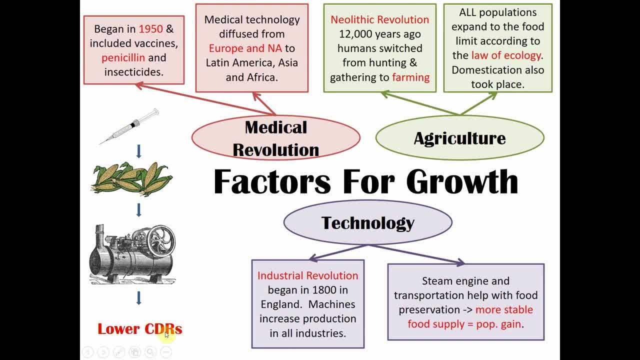 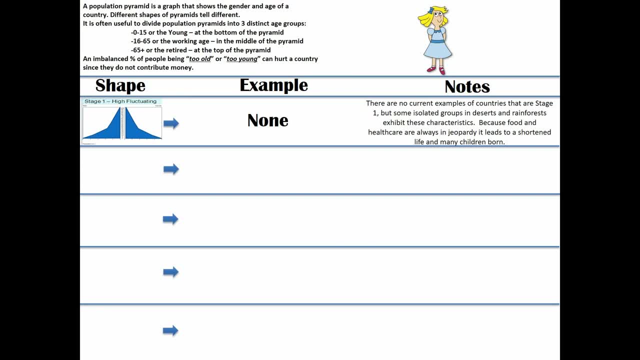 ding a lower child death rate. So let's first talk about How to read these population pyramids. It's basically a representation of a country's population And it splits into three parts. You have the young, which is zero to 15.. Some of y'all are in that, The working age 16 to 65, if you're that age and don't have a job, guess what, Get on it. And then there's 65 and up the golden years: also don't work. 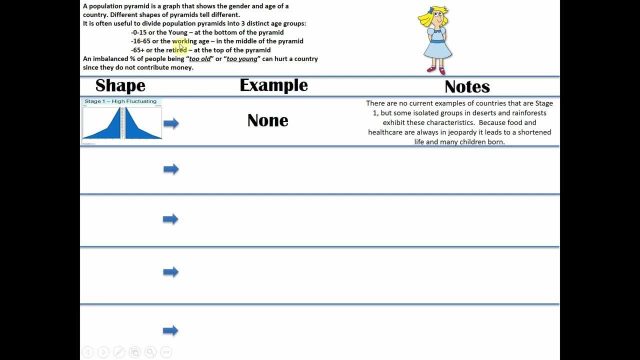 So you'll notice two of these groups do not contribute to the economy and one contributes massively to it. I always tell my students, When things are too old or too young or too hot or too cold, always think of this: Goldilocks. So if there's too many babies in a country, that's bad. 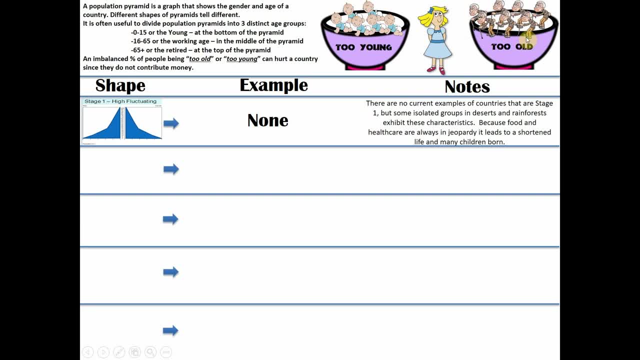 Conversely, if there's too many old people in a country, also bad. Think about it. Surround yourself with too many young people: diapers, whining just like snot and weird just ugh. Right, Too many old people. 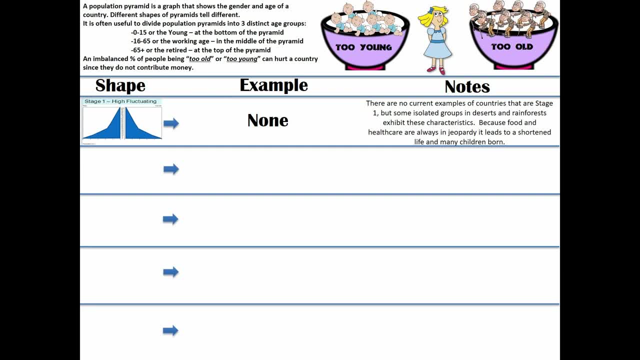 Right. A lot of complaints about soup Tubs, Their back Fluids Right. Both of these are too bad. So what we're going to learn now is how to identify if a country is young or old or in the middle. 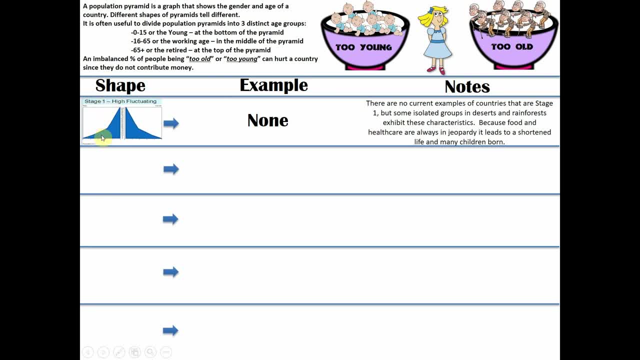 And we do this with these population pyramids. So we'll see the first one. right here is the stage. one country. You'll notice everyone is at the bottom right. You have all these young people, Everyone's down here. This is the vast majority. 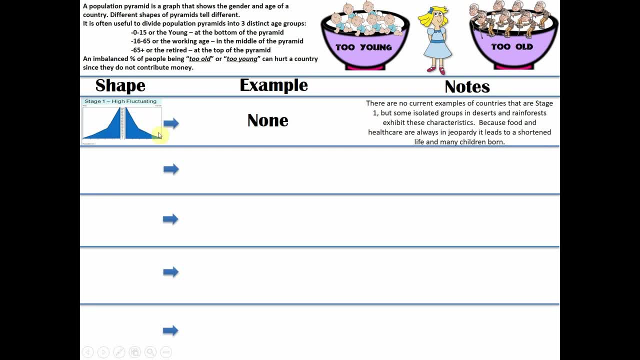 And you have girls on the right, guys on the left, because girls are always right. There are no countries there today And the reason There are so many kids here is there's no preventative prophylactics, no sex education, Just generally. people don't know better. 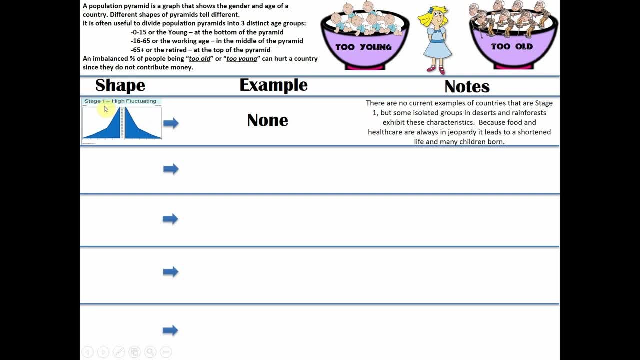 And there's not a lot of old people. You'll notice there's not many old people up here. The reason for that? not a lot of medicine. People live hard lives and they die earlier. So that's a stage. one country. You have an extreme amount of young people. 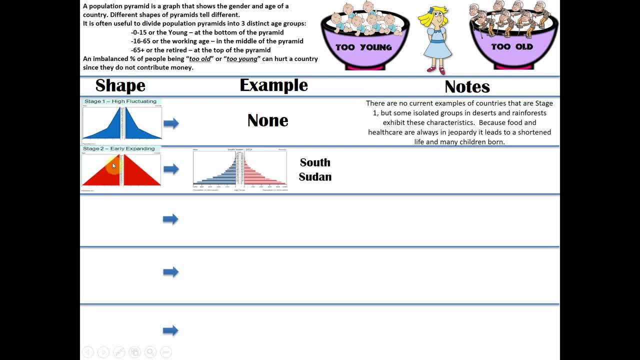 Very few old people And a stage two country looks like this. Now, here's that's. you know kind of what it looks like in a theoretical sense, But here's a real country from 2014,: South Sudan. Notice, there are a lot of kids in this country. 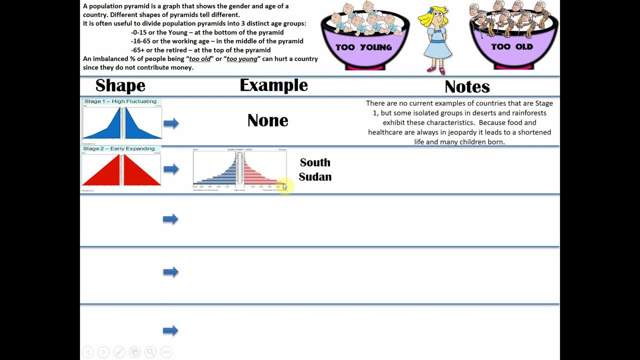 We see down here. from there's 14 and down, We see a large majority of the population, boys and girls, And the reason this country is like that again is they don't live for a long time. They don't have, they have a low life expectancy because of strenuous work. 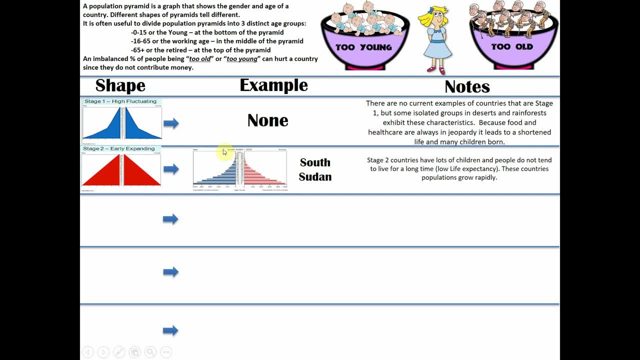 Maybe they have to work with subsistence farms. Maybe they have to work with subsistence farms. They have a lack of machinery and tools and not a lot of healthcare, not a lot of access to medicine, a very high doctor to population ratio. 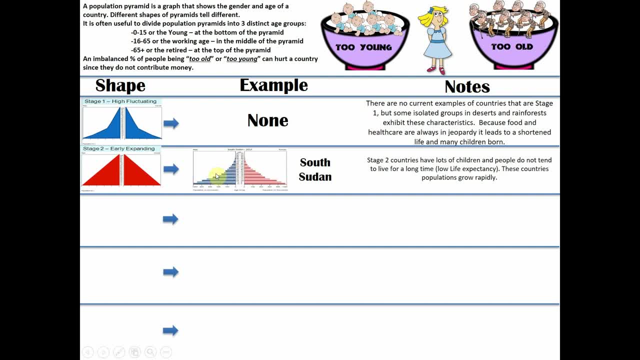 So you can see, because of that you have a lot of kids. It has a ton of population momentum. A stage two country will eventually transition into a stage three country, And Brazil is a good example of this. This one kind of looks like an onion, or those Russian domes. 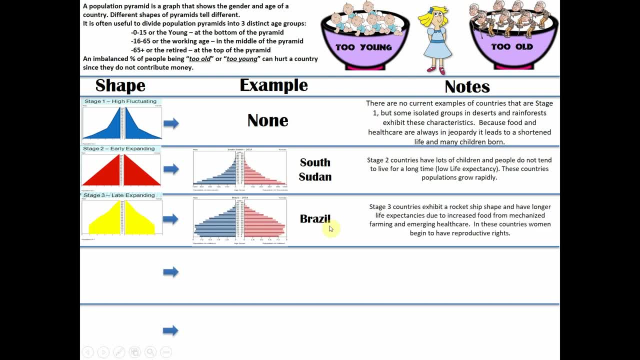 Da In Brazil, we notice has this rocket shape and they have a longer life expectancy. You'll notice there are more older people And all of a sudden we see the younger people starting to wane down here. These lines aren't touching like they were up here. 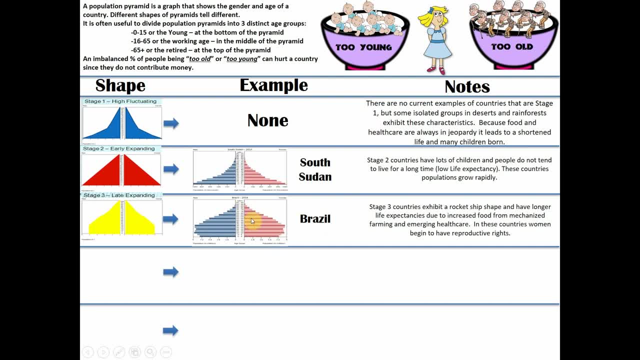 So less children, a little more old people. We notice everything's kind of moving towards the center, and you'll notice in stage three and four a lot of middle aged people like myself, which I think is awesome. In a stage three country, though, they'll have more food for mechanization. 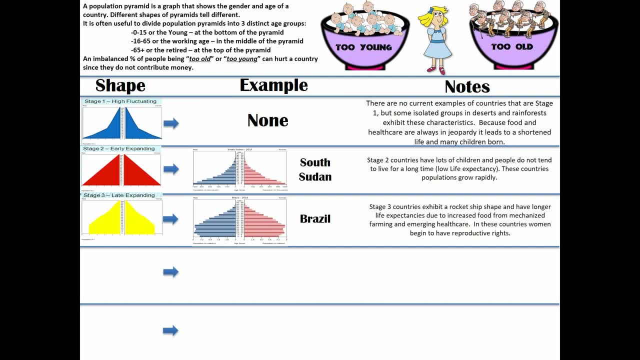 They've industrialized, They've urbanized And you'll notice that in a stage four country like Portugal, it started to look like that. You'll notice the children starts tapering off, They keep climbing with more and more elderly people And we see there's that baby boom. 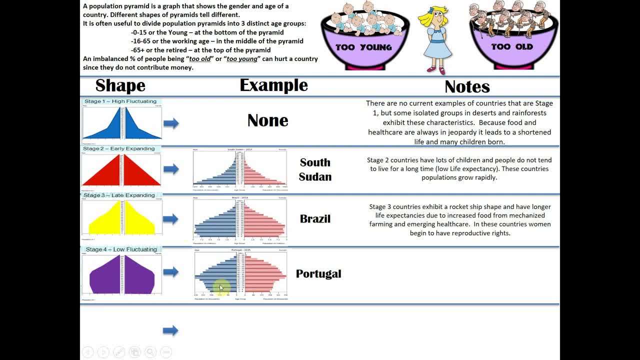 You can watch it go through there, So it's like just keeps moving through. And in Portugal they will eventually hit what's known as ZPG, or zero population growth, because now women are given the right to choose. They are waiting to have children. 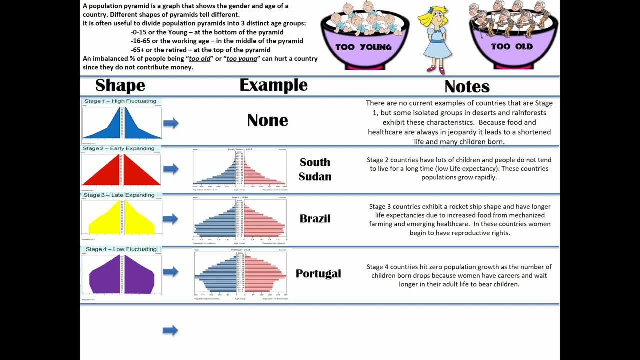 They're waiting to have careers, They're not just going through puberty and having as many kids as possible. They have a lower total fertility rate, somewhere lower than 2.1.. And lastly, you have a country like Japan, And here's Japan's population pyramid. 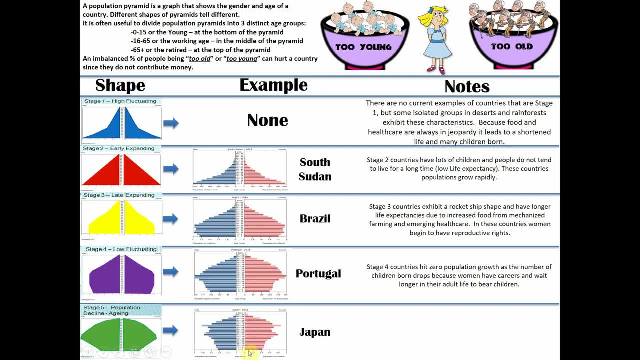 You'll notice an extreme amount of elderly people and they actually have negative growth. So Japan is actually declining or decaying, However you want to say. decay sounds bad for people, but declining And it's mostly due to the fact that people wait. It's so long to have kids because they want to be financially ready or they want to live their best life- Hashtag: you know you do- And they miss their childbearing years, their fertility years, and they can't have as many kids. 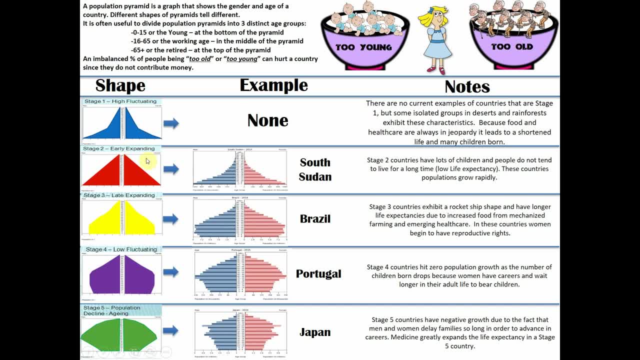 So these one and two, you'll notice a lot of kids, a lot of kids. Stage three: it starts to taper off. Stage four: you have a good bit of balance right. If only you could hold it to stage four. 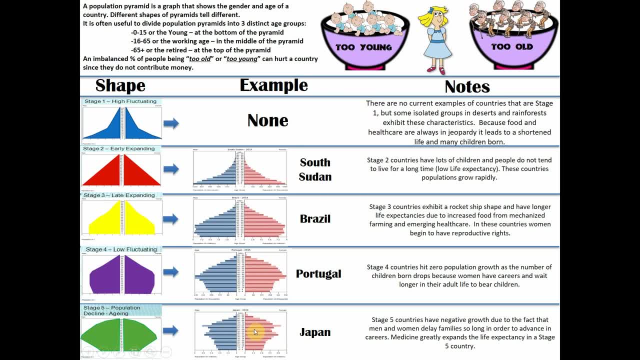 It's not growing, It's not dying, And then in stage five, it's actually in a negative rate. So that is how we look at a population pyramid. So remember it's split: Girls are on the right side, Boys are on the left. 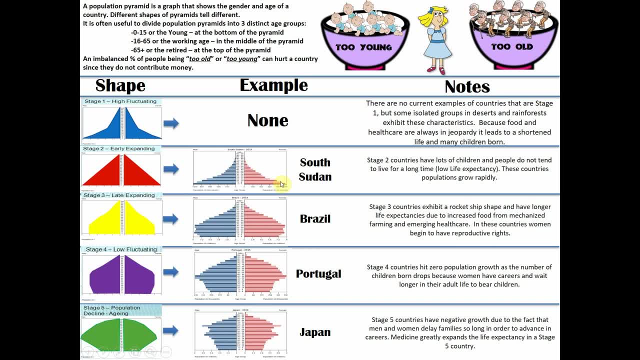 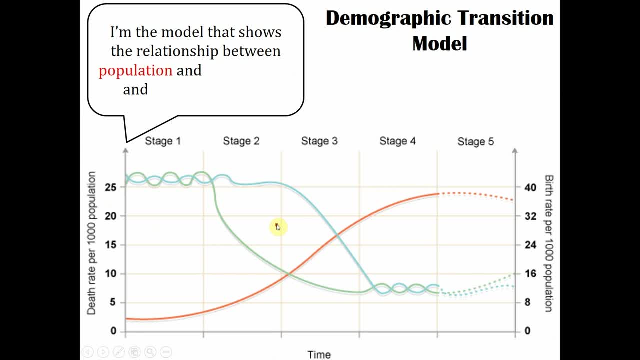 Girls are always right. These are some examples of stage two, three, four and five countries, And over here you'll see some of their notes. So how does that fit into this demographic transition model that shows the relation between population and urbanization and industrialization? 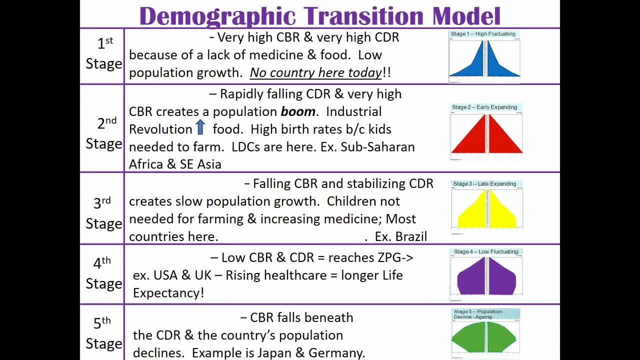 Well, you came to the right YouTube channel because I'm about to tell you kids, All right, sit down. So we've kind of gone over it verbally. I just want to go over it one more time. So stage one has low growth. 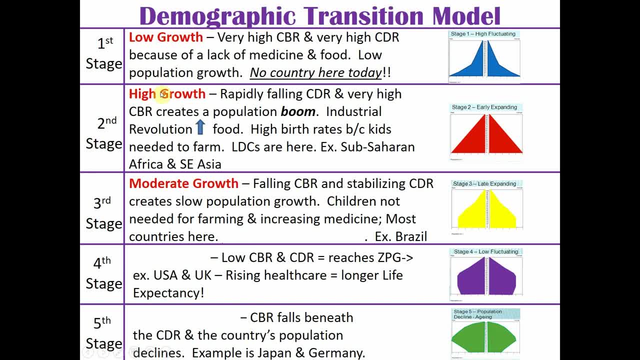 We saw that Stage two has explosive growth, Stage three has moderate growth, Four has low growth again and then five has negative growth, And we're going to look at each stage stage by stage in order to ascertain this. So I've broken it all like this: 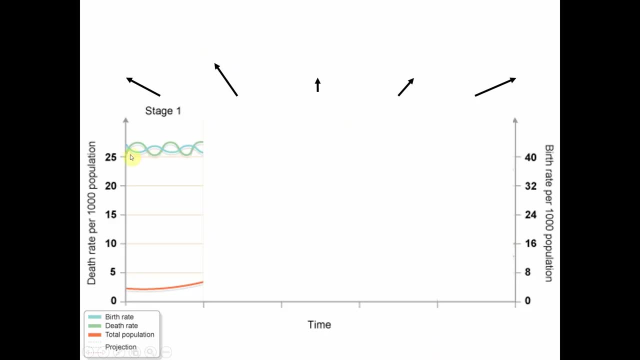 So don't look over here, because when you look at all of it you get overwhelmed. So in stage one we have three kind of factors we're looking at. The blue line is births, The green line is growth, The green line- right, oddly- is death. 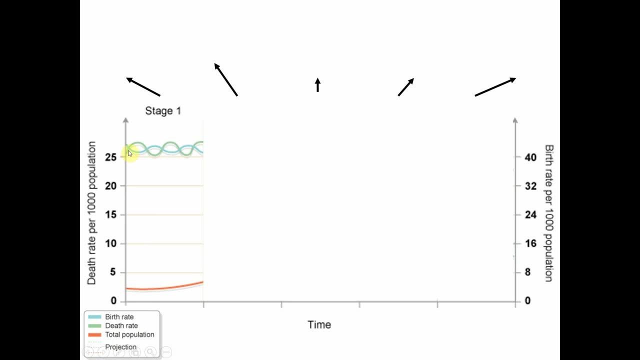 And then the red line at the bottom is total population. So in a stage, one country, there are a lot of deaths and there are a lot of births And you've got to think why, Mr White, Why would that be? 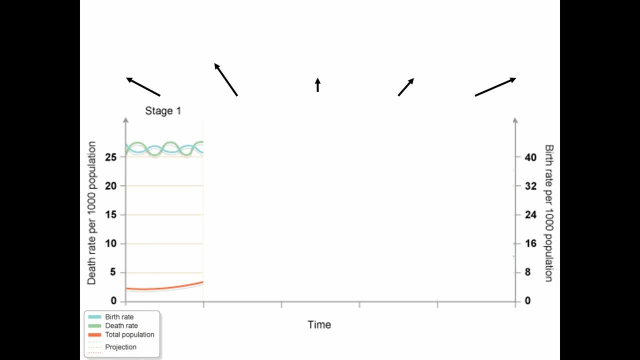 Well, Billy, the reason there's a lot of births is: think about it In a stage. one country they're living out in the jungle, it's tribal, There's no education. There's going to be a lot of births, a lot of hand-holding. 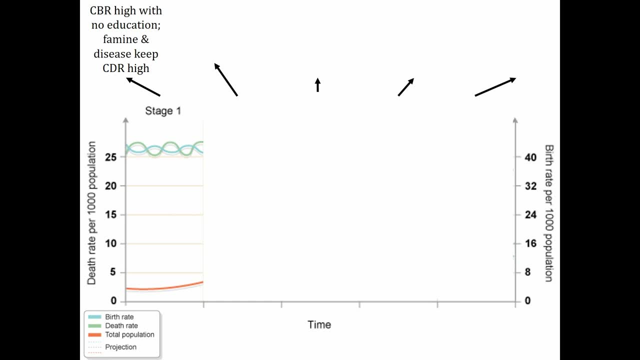 Why would there be a lot of deaths? Well, they don't have modern farming and agriculture, So because of that, we'll notice that this death line is up very high, And so these fluctuate from time to time, based on just maybe there's good seasons, bad seasons. 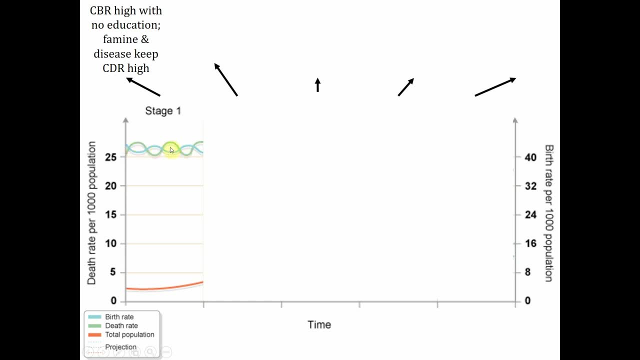 more animals, less animals to hunt, But because these are so close to each other, you have basically a net zero here, which is a bad ISP from the late 90s, But in this case the low population growth- It's slightly growing. 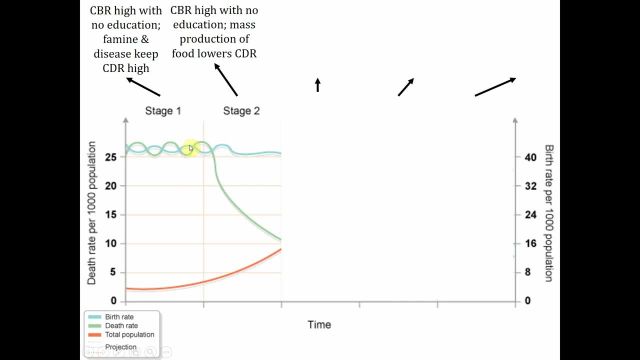 So that's stage one: No countries there today. Stage two: Here's what it's looking like. All of a sudden you'll see these lines that were kind of like flirting and giggling They have now. they are very far away from each other. 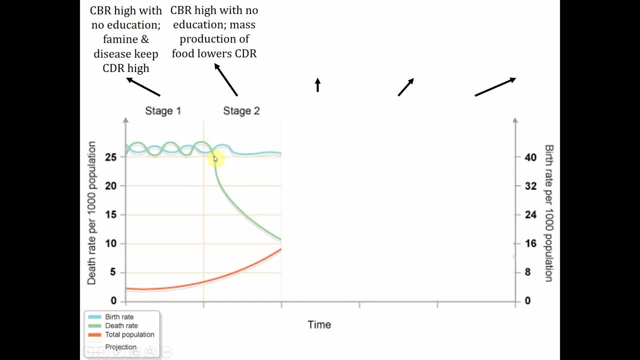 So you still have an extremely high birth rate in stage two country, But what has fallen rapidly is the death rate, And that's mostly because there's some mechanization, There's a little bit of industrialization here And there's more food available. 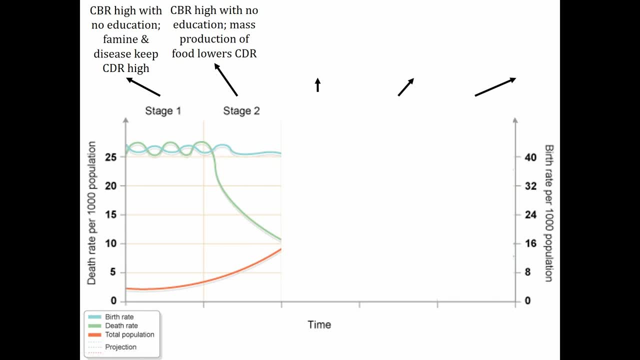 And we all know, when there's more food available, there's more people. Think about it, right. If you just yell out free pizza, you're going to make some friends, right? People you don't know are going to come find you. 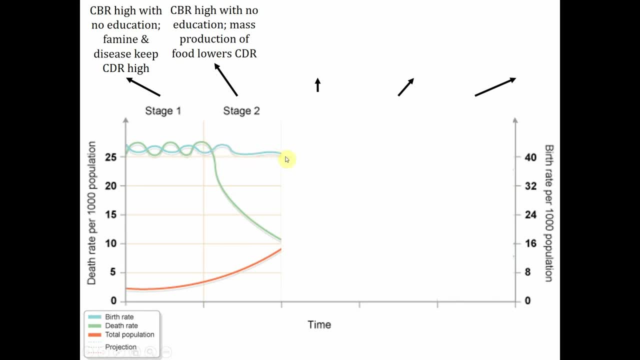 So why is the blue line so high? Well, in a stage two country, women still don't get educated. That's the biggest reason that we'll decide where this blue line will go. Women are devalued, Women aren't expected to work. 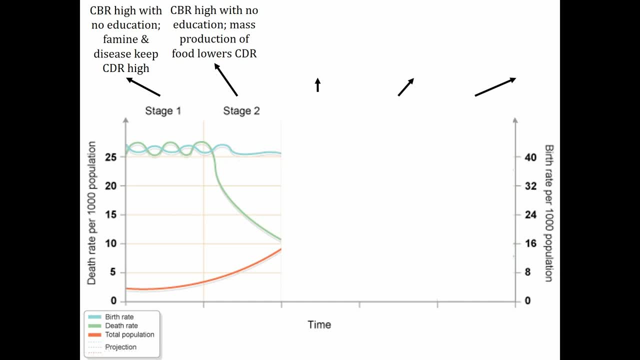 They're just expected to give birth In a stage two country. a woman could have upwards of 13 or 14 kids on average in some sub-Saharan and Southeast Asia. So we see that because of that right, this high birth rate and this plummeted death rate, 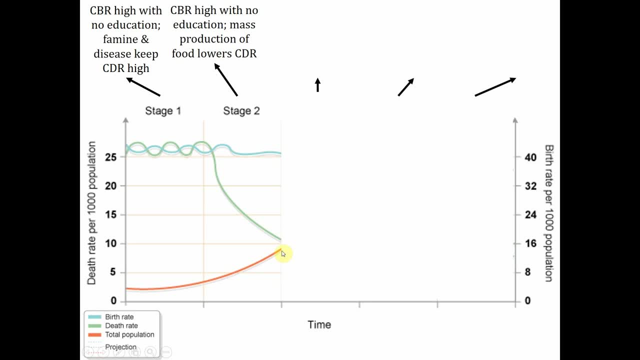 we see that the red line will curve sharply up. We get a new slope. Stage three: we'll notice the red line continues and then it starts to soften And we'll notice the biggest change in stage three is the green line is still kind of where. 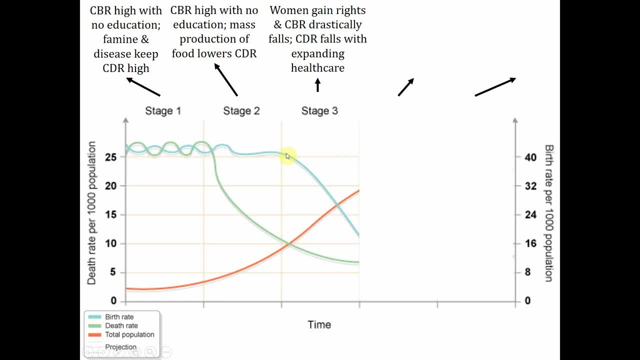 it has been with this death rate. But now all of a sudden the birth rate, or this blue line, plummets greatly. And the biggest reason here is: women gain rights. So in a stage three country women start to demand all their rights. 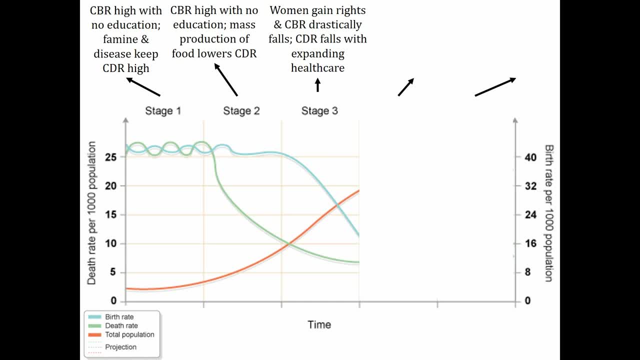 Whether it's equality, pay, childbearing, productive rights, educational rights. And when that happens, look out right, because you're going to have much lower birth rates. Lower birth rates mixed with already low death rates means that the population will slow. 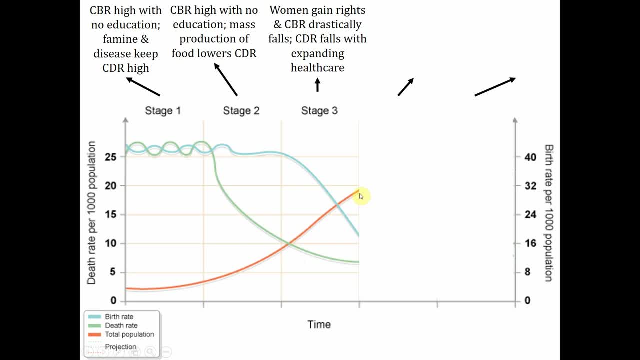 down. So you have like the brakes are getting hit. in stage three, towards the end, We can see the red lines starting to taper off. here, In a stage four country, you'll hit what's known as ZPG towards the end of it, which. 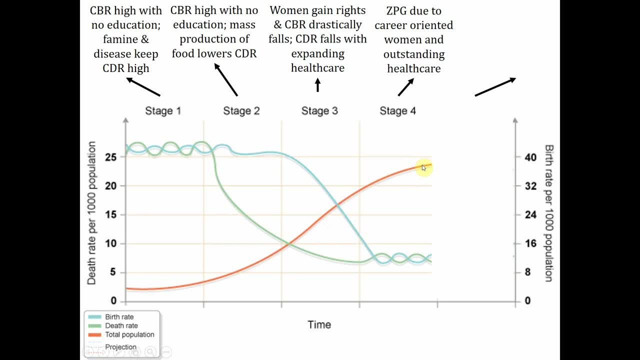 is zero population growth And it's a continuation of stage three here, because you still have women choosing. You'll notice that these lines have now kind of interplayed again And you have better health care. You have women focused on their careers and starting families. much, much later maybe, 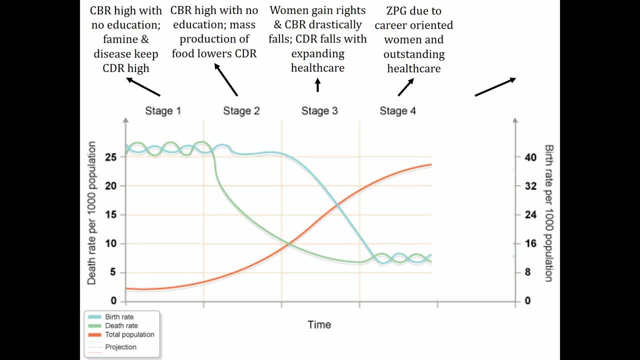 30,, 35. And you know, at that point women aren't able to have children, And this used to be where the difference was. The demographic transition model quit with stage four, But recently some countries have gone into negative growth or decay. 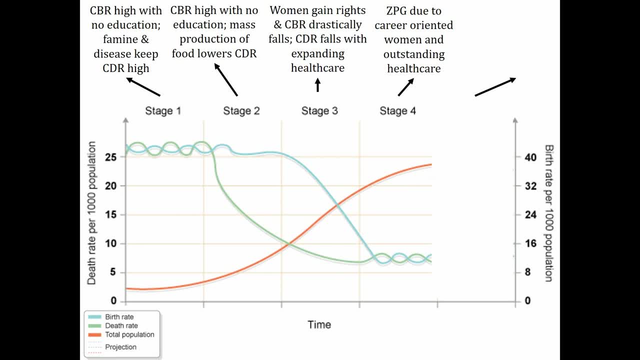 And so some geographers and demographers have put in this fifth stage. And the fifth stage will state that the country's total population will grow negative because- and at this stage we'll see- that the birth rate will fall below the death rate. Now you got to remember. it'd be nice if no one ever died, but that's the rule. 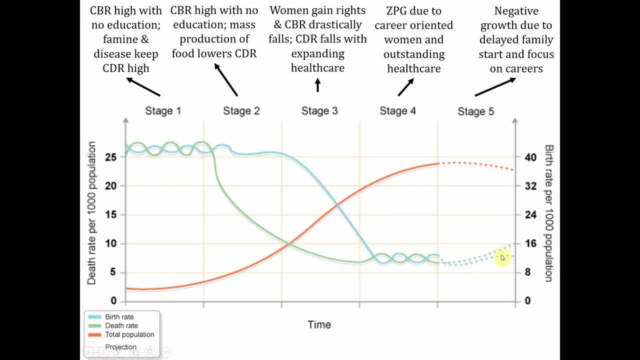 So death can't ever get done here. Births can get lower and lower because, again, you have people focusing so hard on their careers that they don't think about OK, well, what about posterity? or family or children? So all of these together make up what's known as a demographic transition model. 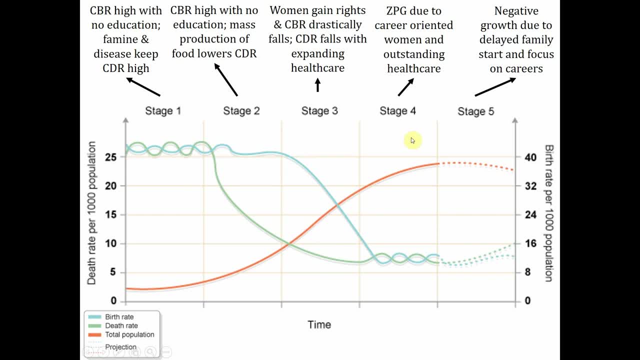 So, as a country is moving through these different stages, there's different variables playing. Maybe there's women getting rights, Maybe there's industrialization, Maybe there's breakthrough in medicine, And all of these changes will make the population shift up or down. 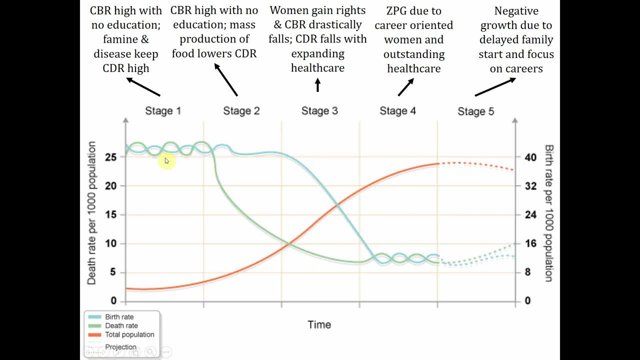 So I hope that helped explain this demographic transition model, Because if you look at it, it's one big graph, It's confusing, It's scary. I was going to draw it And I was like wait, Mr White, you can't draw. 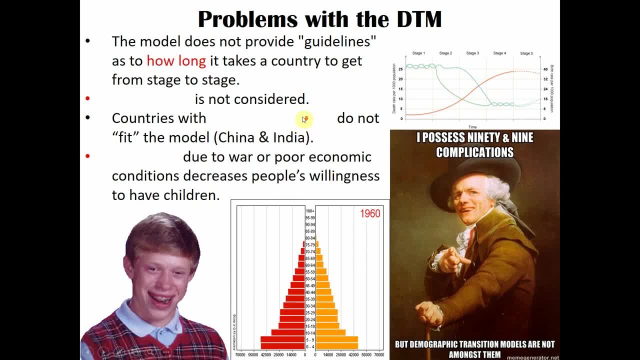 You're stupid, right, But there are problems with the DTM. It never tells you how long it takes to get anywhere, It does not consider it immigration, And if you're a country like China or India that have these severe population problems, 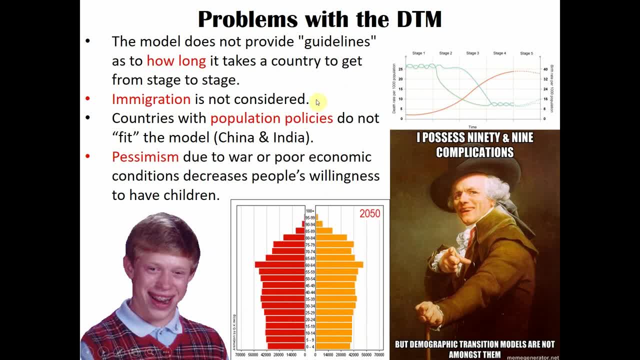 it doesn't have a real good answer And also if there's economic downturn or war it can't account for it. But this right here is a population pyramid of Japan. Notice it's going through all the stages And you'll see that those kids born in 1950 are getting older and older. 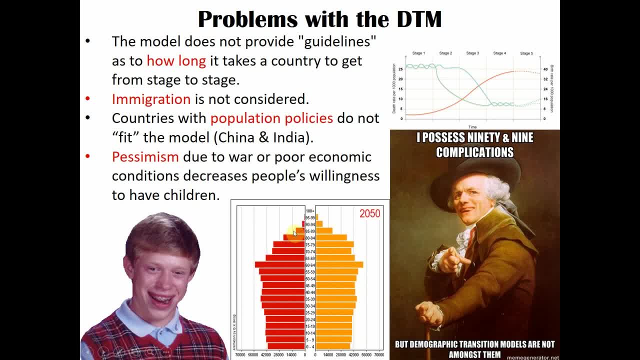 Now they've passed to modern times And you can see it go from a stage two to a stage five. country right before your eyes And just see it exploding in growth. Stage two Now it's going to stage three, It's going to stage four now. 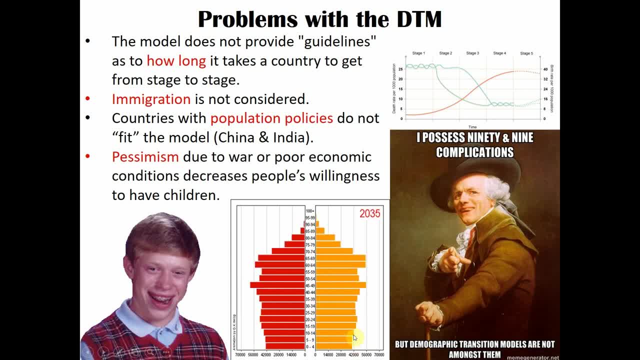 It's starting to get all those shapes And if you can just identify the shapes and know some of the causes behind them, that'd be very helpful on the AP exam in May that you're going to get a three, four or five on right. 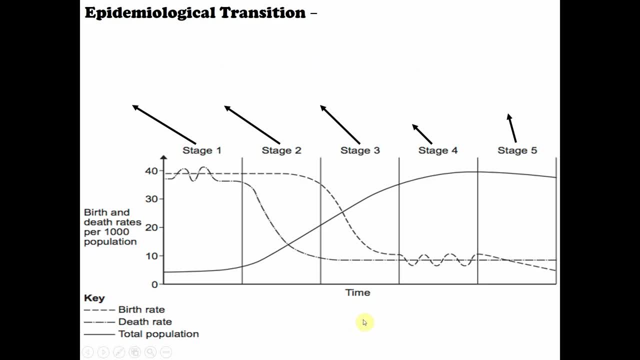 Speaking of May, that'll be the end of the class, But this can also be used to state how do people generally die in the DTM, right, This is normally a bright pod or YouTube happy topics, Right. But if you look at the epidemiological transition, each stage has a typical way people die. 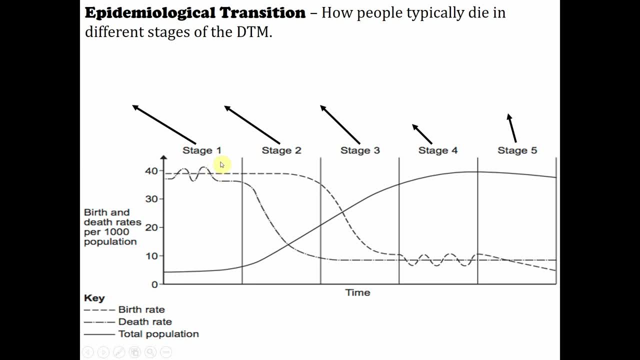 So in a stage one country- which not any in here, but you could say some tribes that live in some remote places- they'll die of famine or widespread diseases because they don't have the ability to mass produce food. In a stage two country, people generally die of widespread diseases like a cholera. 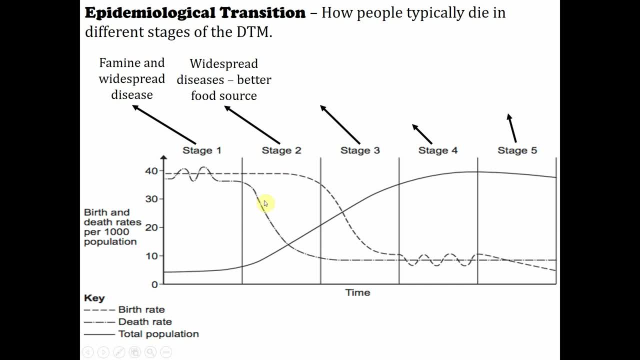 Not famine, though, because they have better food because of the industrial revolution. So that's where You know you get these larger populations. people start living together and a sickness can break through. In a stage three country, you have what's called degenerative diseases. 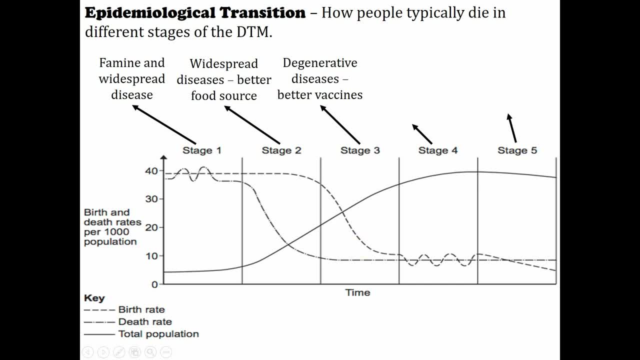 Now people are dying from their organs, physically giving out of gas. right, People aren't going to die of famine or disease anymore. So those are the number one killers. in stage one and two And stage three and four you have degenerative and then four delayed degenerative because 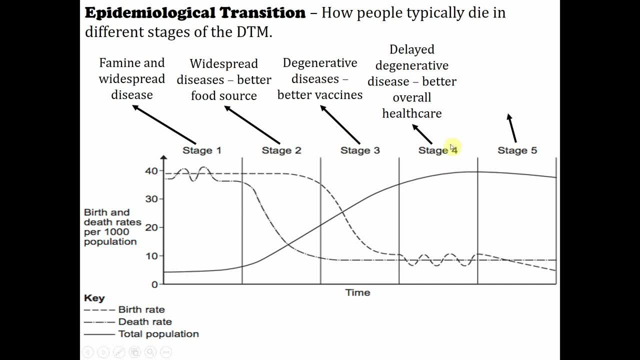 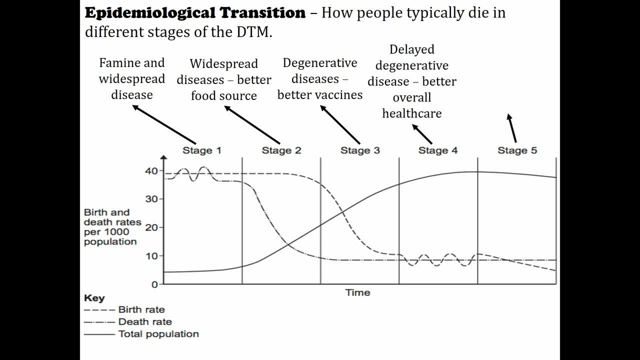 little cases that say Monday, Tuesday, Wednesday, Thursday and they pop them open. They got to take all the pills, right? They take all those pills to delay their degeneration of their organs. If they do not take those pills right? 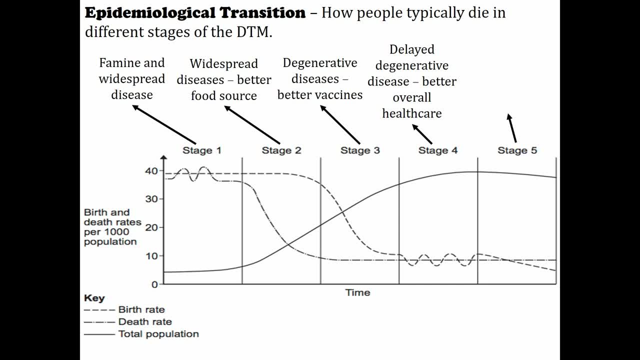 They wouldn't make it that far. And in stage five, since we don't know that much about it generally, people are going to die of what's known as antibiotic resistance. Just the diseases start to evolve or change So how we've always treated them. 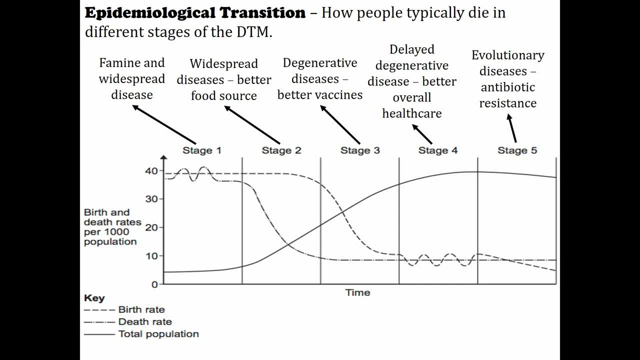 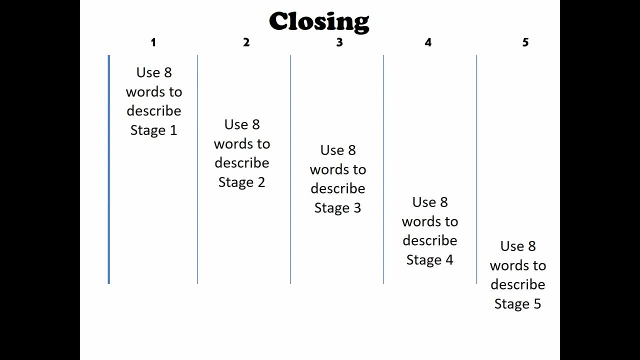 this constant method we've always taken. it's now no longer effective and there's change occurring, So it's something that we don't quite see. So this is how generally people will die. In my class, I usually make my kids go around and write down each of these stages in, you know. 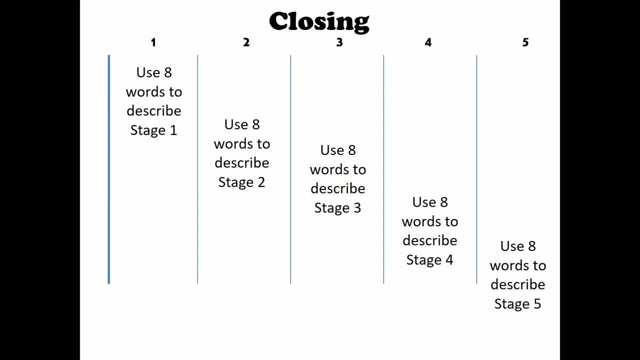 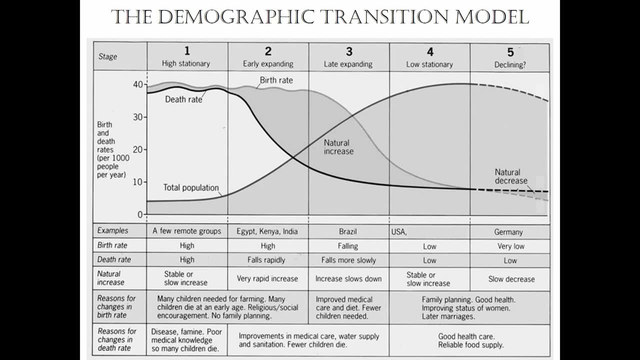 eight words. But for you guys, since I can't do anything, I can't make you do anything. I'm just going to make you stare at this And if you memorize this and just stare at it, talk it through, explain it to your dumb little brother or sister, tell your you know.